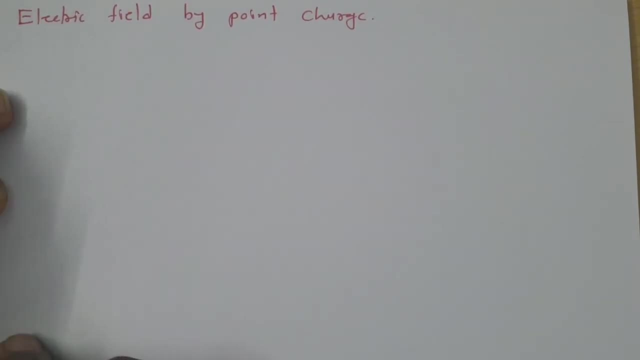 Welcome to electromagnetics playlist. Here in this session I will be going to explain you electric field by point charge. Now see in previous session I have already explained you Coulomb's law and in Coulomb's law I have explained force will act in between two charges. 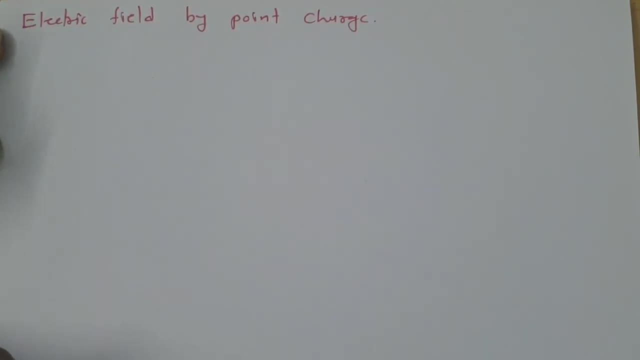 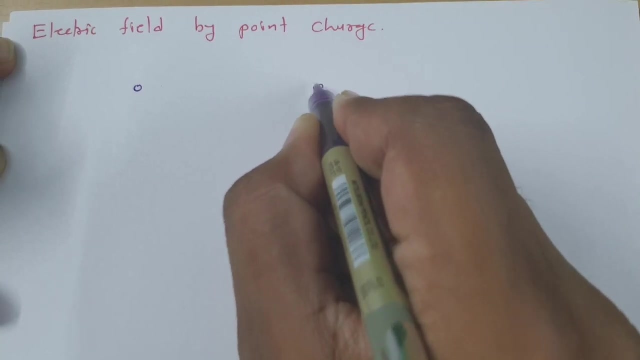 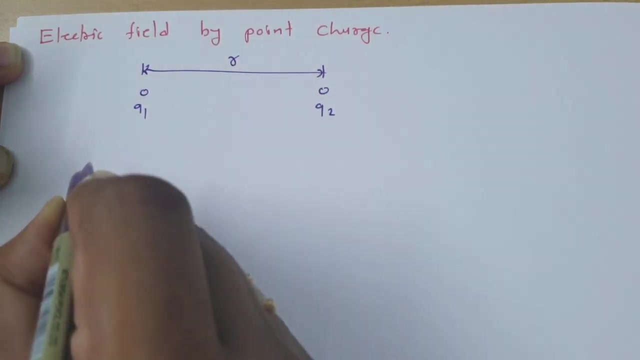 and in that we have already seen the direction of force. So if I just give you a quick review of that, then see if two charges that is given to you, let us say q1 and q2, and if these two charges are reported by distance r, and if I consider first case, q1, q2 greater than zero means 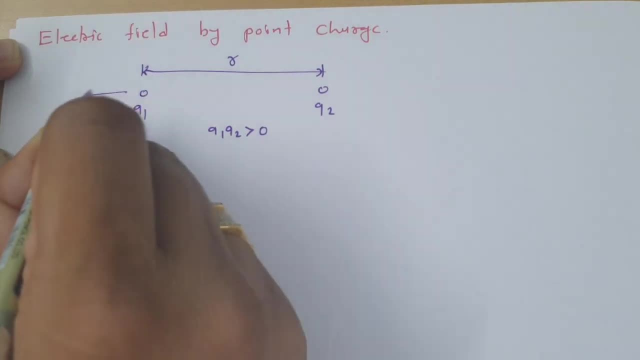 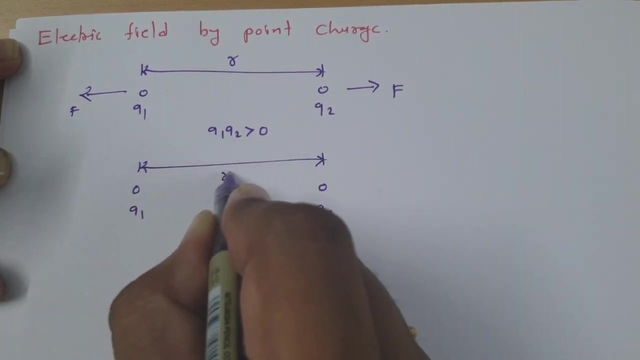 polarity of these two charge is same, then there will be repulsive force which will act in between these two charge. and if you have two charges, let us say q1 and q2, and if both are separated by distance r, and if these two charges are having unlike polarity means, 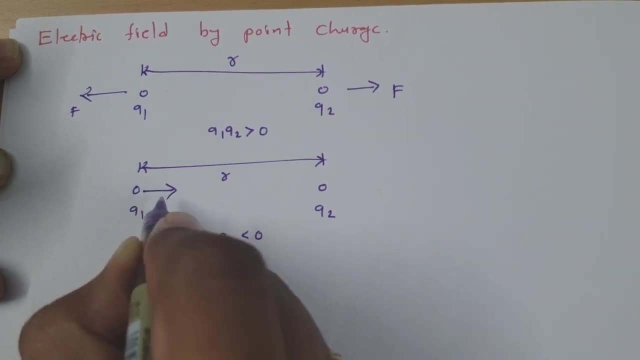 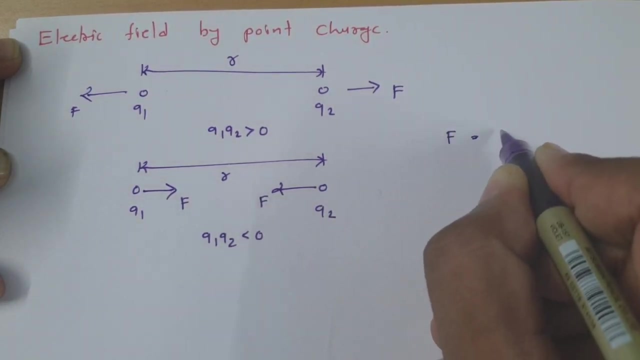 q1- q2 is less than zero, then you will be finding there will be attractive force which will happen, and magnitude of this force that we have calculated, that is 1 by 4 pi, epsilon, 0, q1- q2 divided by r square. So there should be equation. 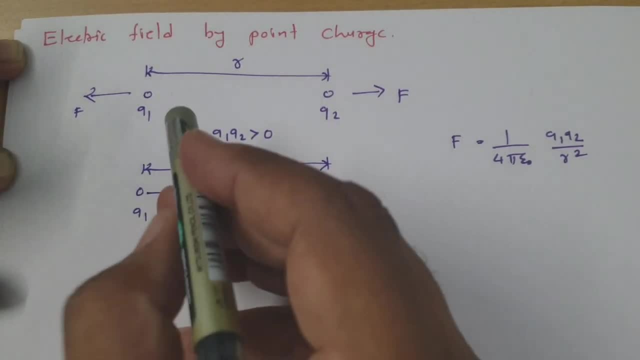 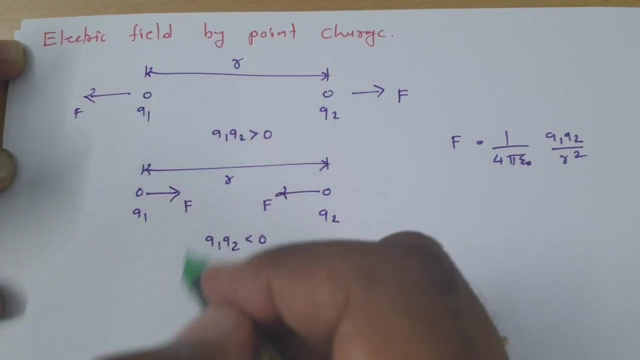 like how this force is acting, like what is there in between these two charge, which is resulting force on q1 as well as on q2 because of each other. So this force is acting because of fields and that field is being referred as electric field. So there must be some field because of q1. 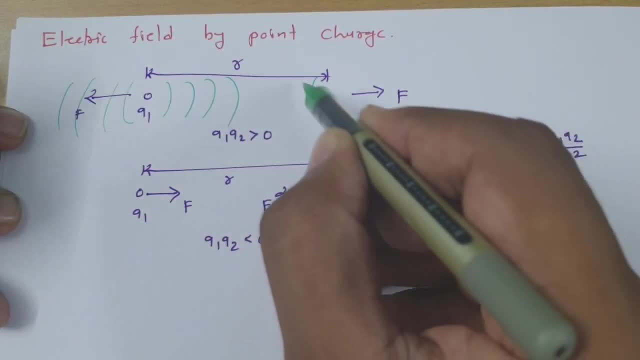 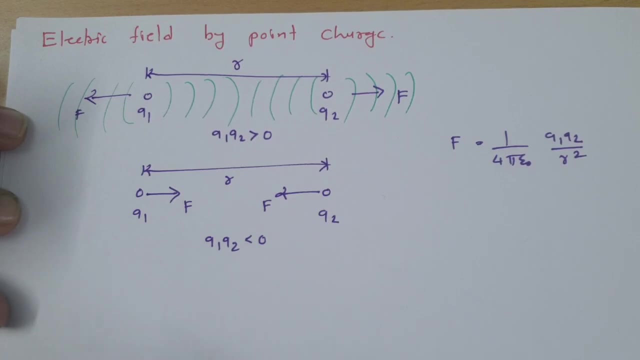 there must be some field because of q1 as well as there must be some field because of q2. And those field is resulting force on each other and that field is referred as electric field. So let me define this first. See electric field that is referred as amount of force. 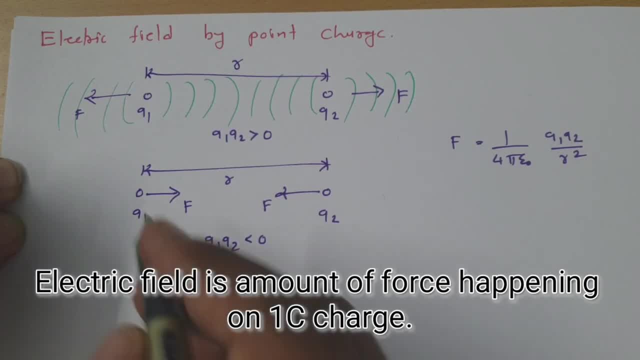 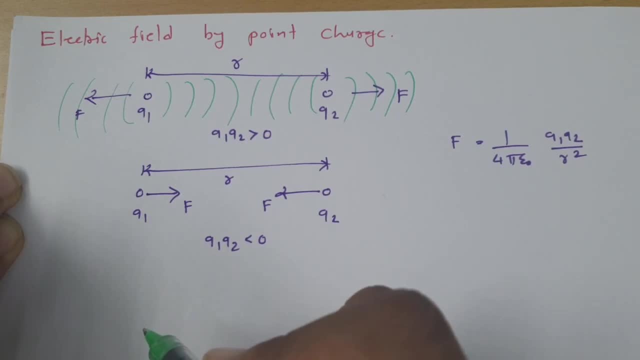 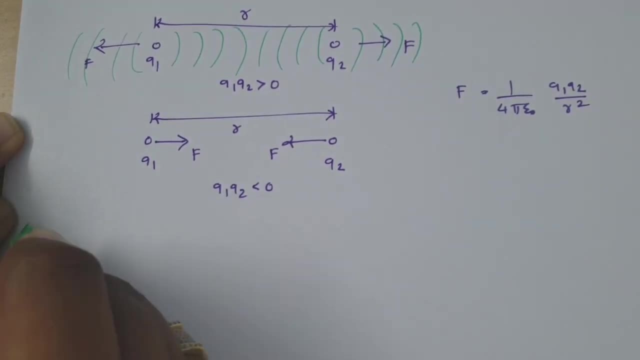 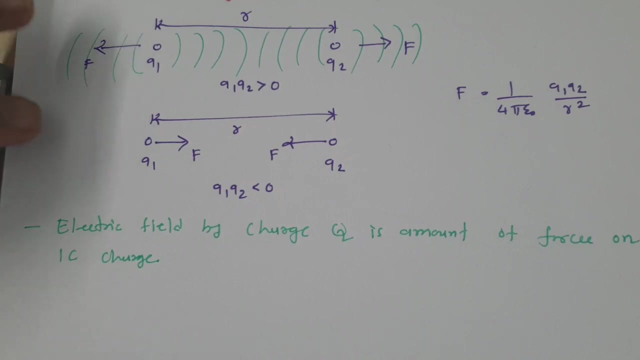 happening on one coulomb charge. So if i want to calculate electric field because of charge capital q, then electric field given by charge capital q is amount of force acting on the one coulomb charge. So let me write it first. So see, basically, as per this definition we 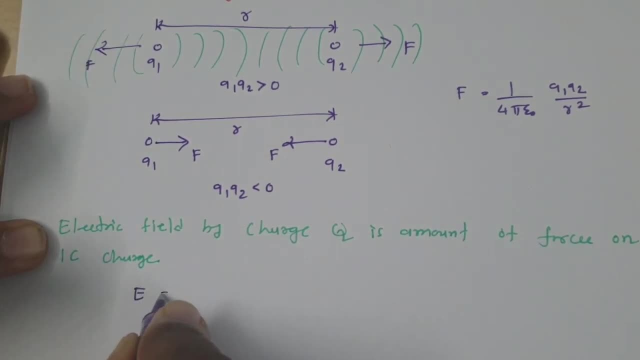 can say electric field, that is equals to force divided by charge. and if this small q charge, that is one coulomb, if this small q charge that is one coulomb, then force is equals to electric field. that we can say. So, as per this basic definition, this electric field. see, if I say 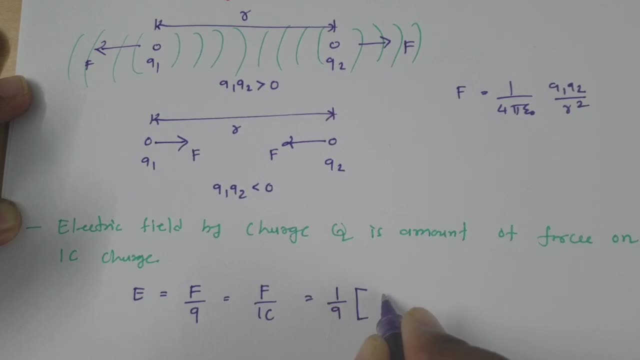 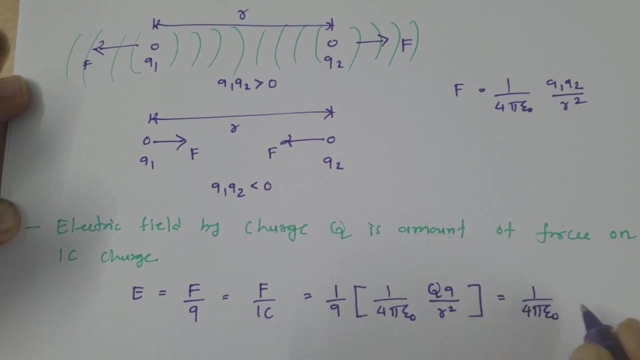 1 by q and into force. that is 1 by 4 pi epsilon 0 capital Q. small q divided by r square, then this small q that will get cancelled and electric field will be 1 by 4 pi epsilon 0 capital Q by r square. 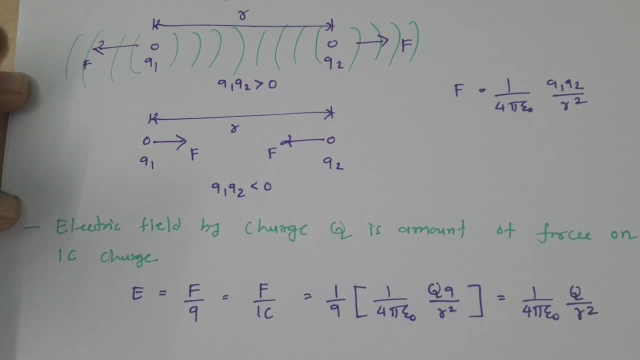 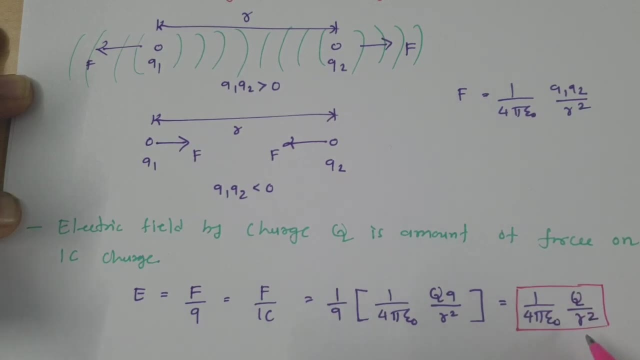 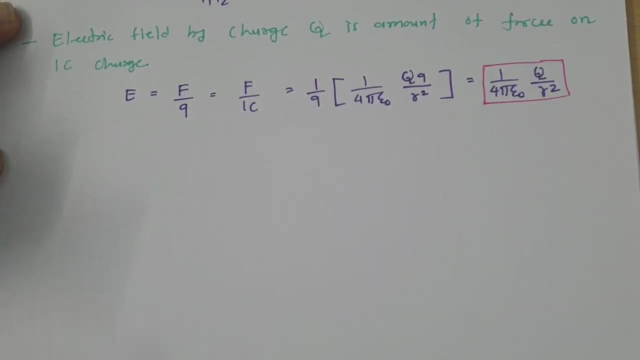 So electric field magnitude, electric field magnitude that is 1 by 4 pi epsilon 0 into q by r square where q is charge and r is distance from capital Q charge. So let us try to understand this how that is happening first, and then I will show you by direction how it is happening. So if we have positive charge, 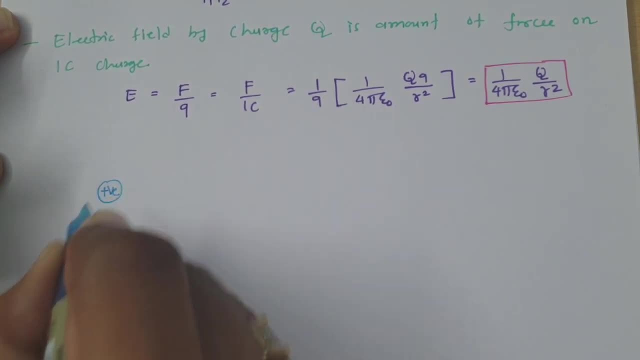 so let us consider a positive charge. So see, for the case of positive charge, you will be finding electric field that is happening in outward direction. So I am just showing you direction right now. later I will show you how to calculate this. So first we need to understand this: if we have positive charge, then electric. 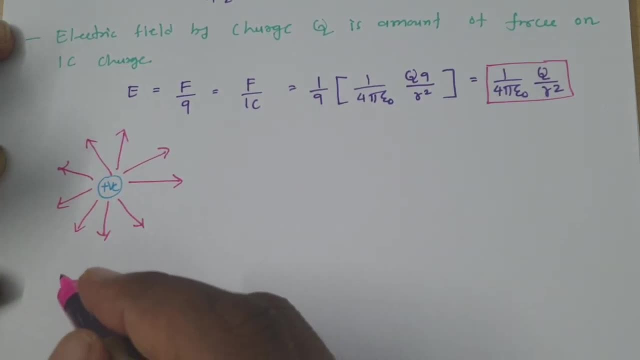 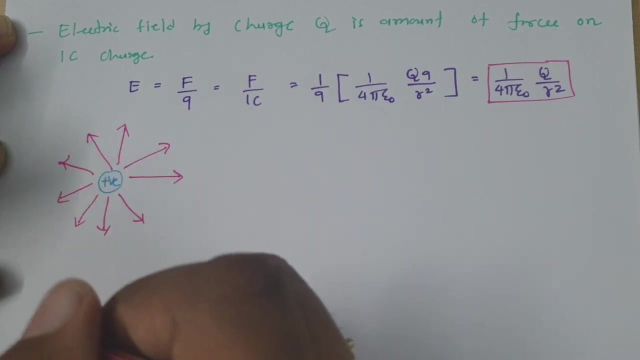 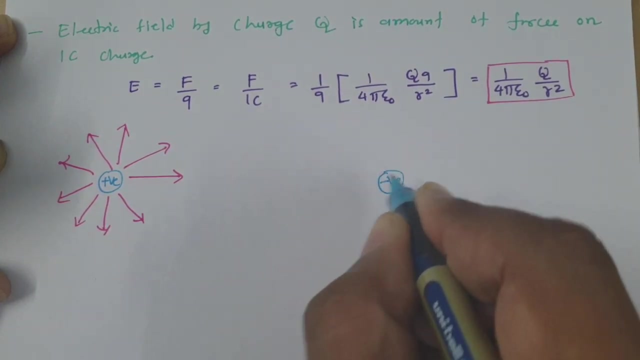 field that will be in outward direction, radially. So if you have positive charge, then electric field will be in outward direction radially. If we have negative charge? if we have negative charge, then you will be finding electric field that will be in inward direction to this charge, radially. So you 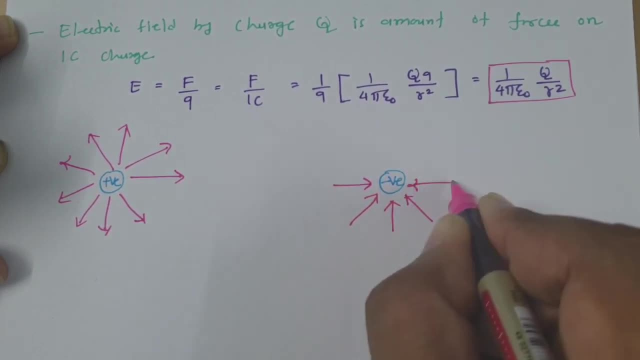 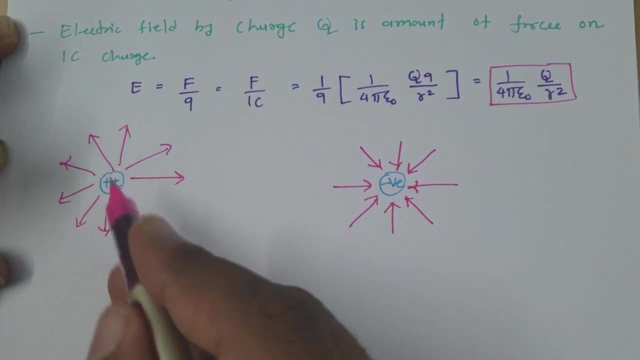 will be finding direction of electric field that is happening inside of this charge. So if you have positive charge, electric field will be in outward direction and for negative charge, electric field that will be in inward direction. So let me write this statement that is very important. 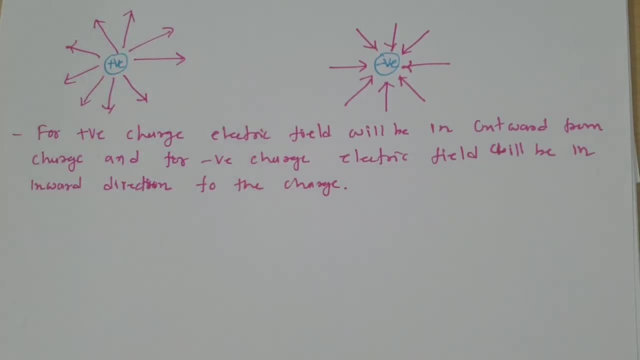 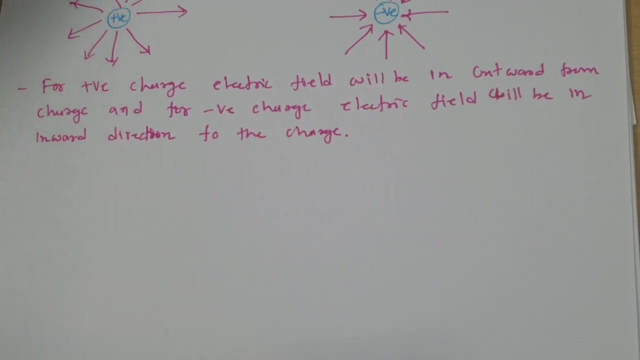 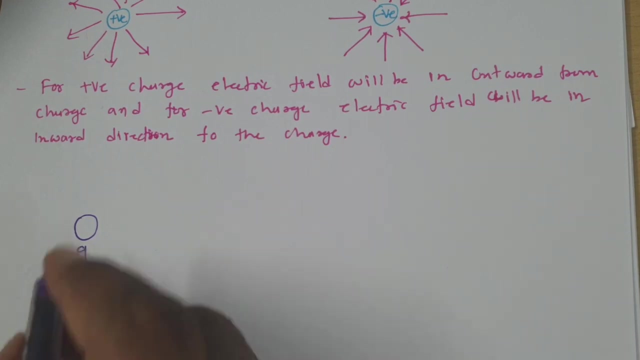 Now see, let us try to understand how to calculate electric field with respect to direction. So see, for example, if I say I have one charge over here and let us say this charge that is capital Q, sorry, positive Q, right, So this charge is positive and its magnitude is Q, Then what will happen? as this: 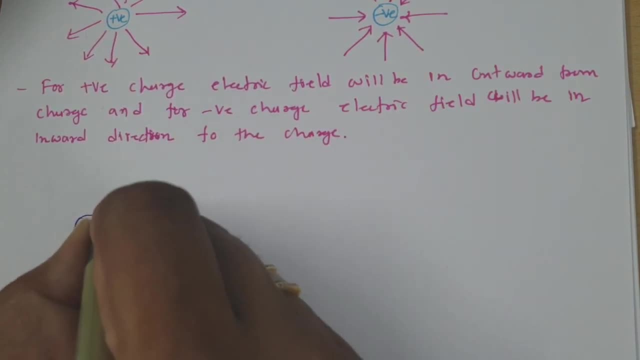 charge is positive, what will happen? electric field that will be in outward direction, Like this. Alright, as this charge is positive. Now, if I consider this charge that is there at origin, so right now I am considering this charge that is there at origin. So, as this charge that is there at origin, 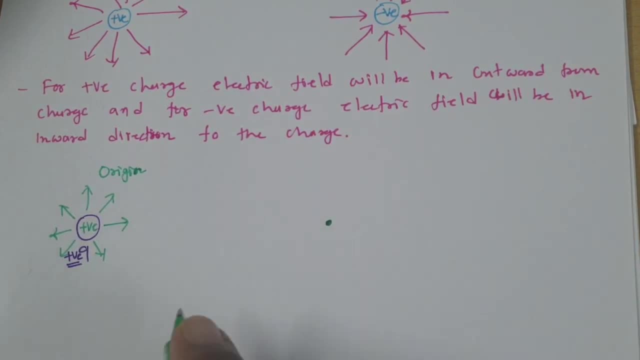 if I want to calculate it, I need to calculate: is��ol q90, calculate electric field over here, then what will be the direction at this point? that direction will be in this direction. that direction will be in this direction. and if we say this distance is r, then electric field over here, that will be E. is equals to 1 by 4 pi. epsilon 0 into. 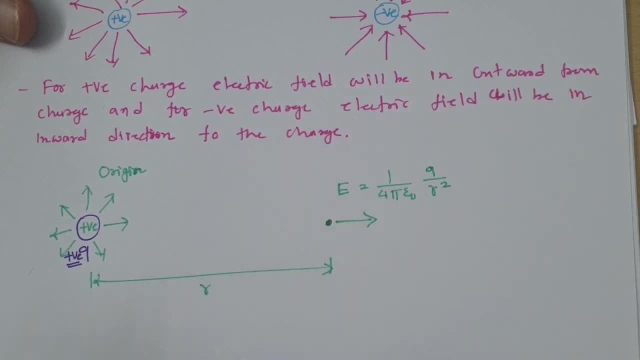 small q divided by r square. and if I want to calculate this with respect to direction, then I need to multiply for a direction. I need to multiply this with unit vector r. so here, if I say this point is located by unit vector r with respect to origin, then electric. 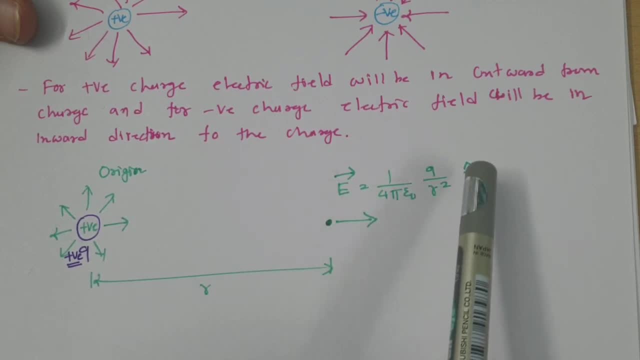 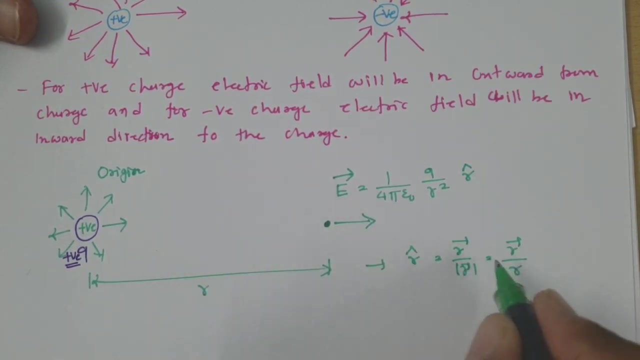 field, that is 1 by 4 pi, epsilon 0 into q by r, square into unit vector r. now see here what is unit vector r, so unit vector r here. unit vector r, that is vector r divided by magnitude of vector r, so that is vector r by r. so if you place this in this formula, 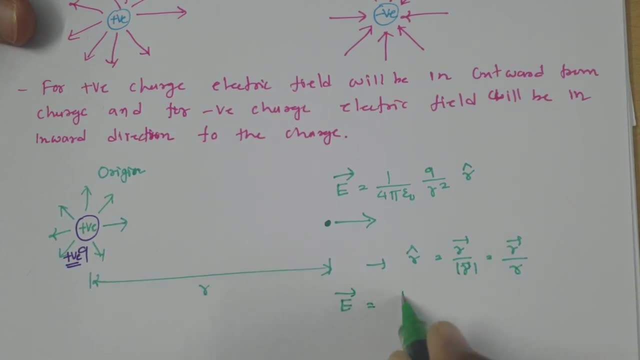 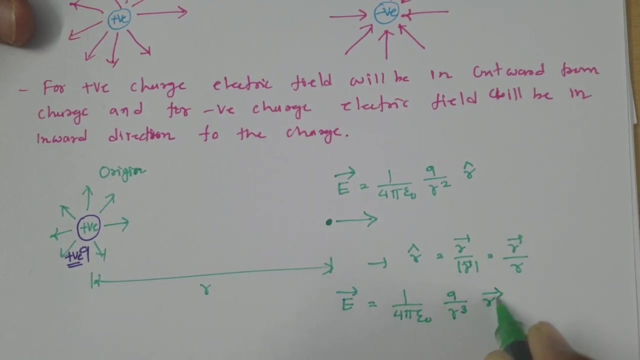 then you will be finding electric field that will be 1 by 4 pi. epsilon 0 into q divided by r, cube into vector r. now see why I am writing this. the reason is I have seen students are finding some difficulties when they write equation like this. they are saying: like in some books it is written as per: 1 by 4 pi. 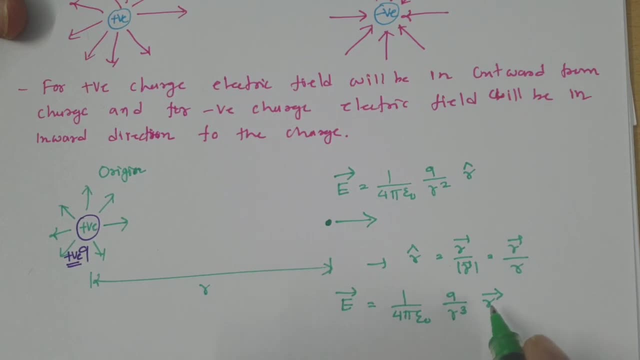 epsilon 0 into q by r cube, into vector r. see, here I have written vector r, so here it should be q by r cube. if I am writing that by direction, q by r square, in that case this should be unit vector r. so this is what one basic difference that one can. 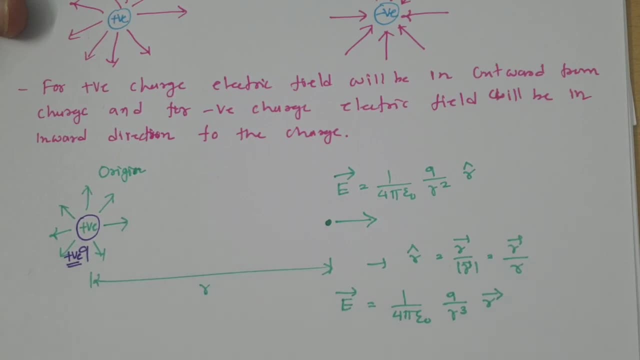 find right. and when you want to calculate magnitude, then we can calculate magnitude as per this formula: 1 by 4 pi epsilon 0 into q, by r square and for direction we need to multiply unit vector r with this. and if you have formula in terms of vector r, then this: 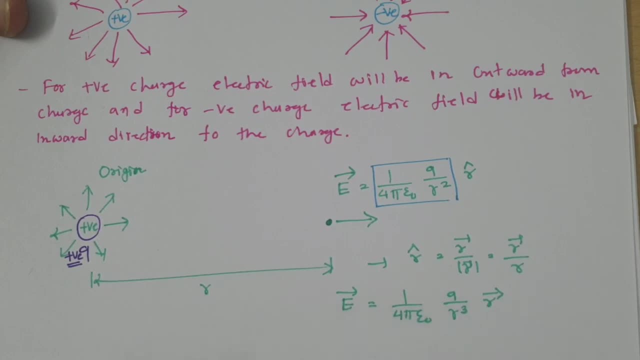 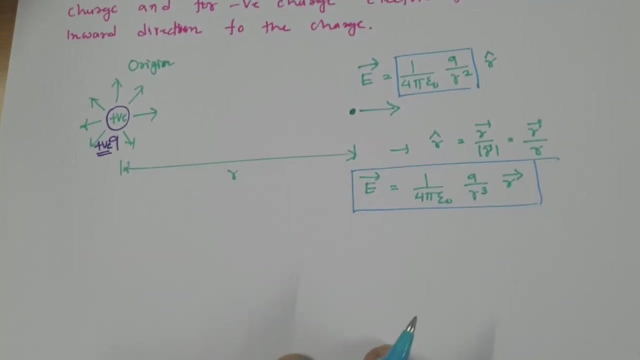 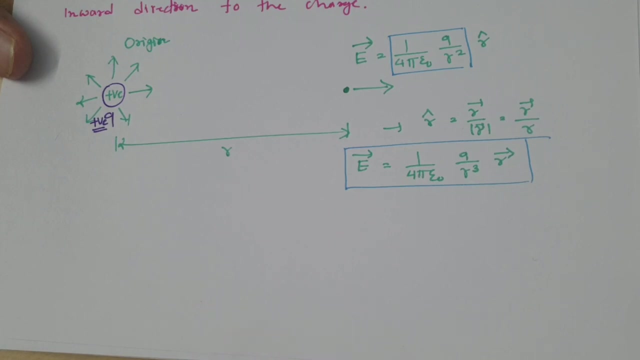 formula will be 1 by 4, pi epsilon 0, q by r, cube into vector r. so this is what we need to take care of when we calculate examples, Thank you. Now I will show you what will be the direction of force under electric field. right so for. 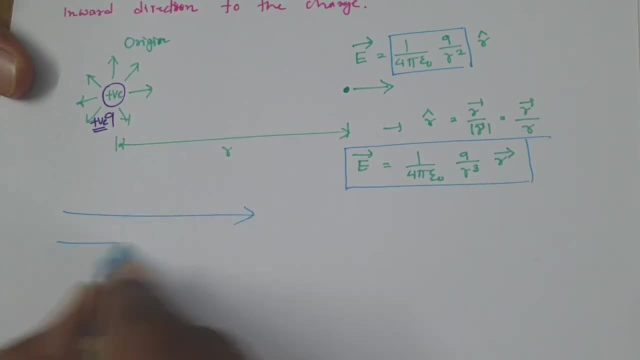 that if I show you electric field which is happening in this direction, let us consider electric field that is happening in this direction, right, and in this electric field, if I place positive charge q- So as if I place positive charge q will be finding force will happen.